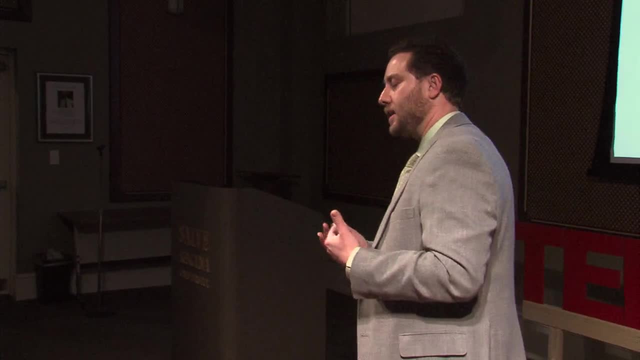 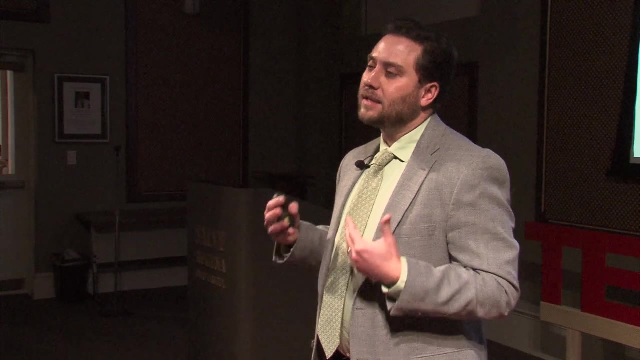 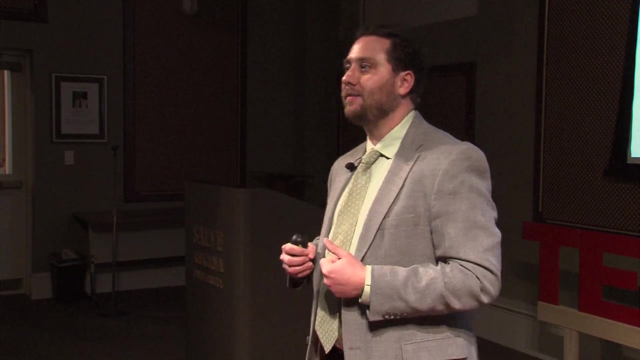 The second reason I wanted to talk about him, or at least begin my discussion talking about him, is because this is the first mammalian species, at least as far as we know, that's gone extinct, primarily because of climate change. Will it be the last? Probably not. In fact, there's probably some that have already gone extinct that we haven't quite identified yet. 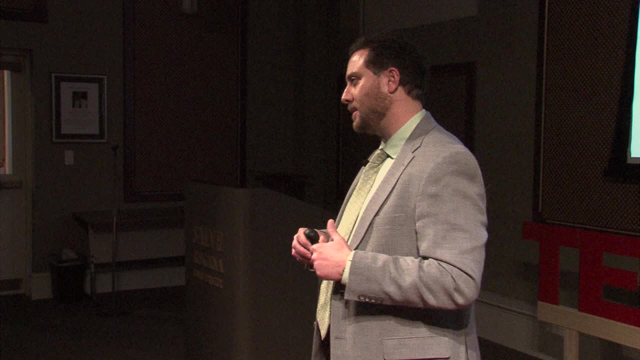 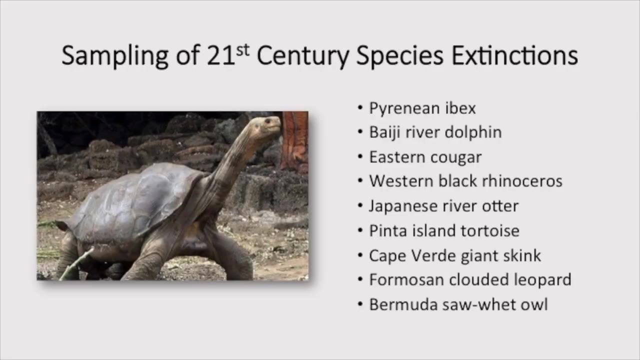 But basically what happened is this was a very low-lying species and its habitat was more or less flooded by rising sea levels, by the Great Barrier Reef. Now species extinction is occurring at an incredibly fast rate. This is just a sampling of some of the species that have gone extinct just since the year 2000.. 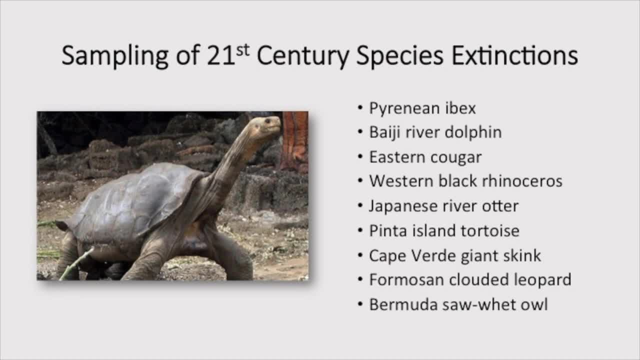 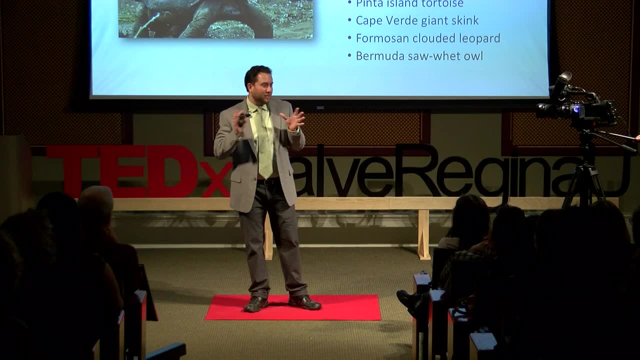 These are the more sort of charismatic species that have died off. This is an image of Lonesome George, who was the last Pinta Island tortoise- At least we thought he was. There may be hope now. We might have found some other ones. 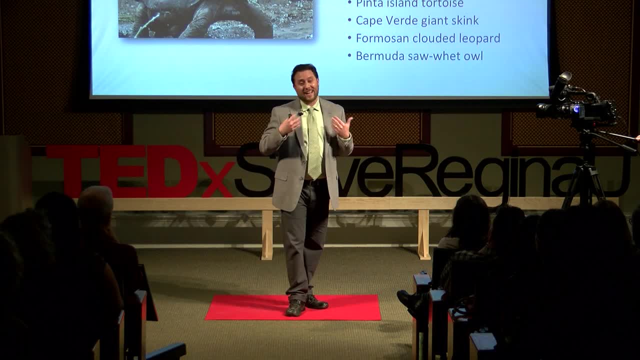 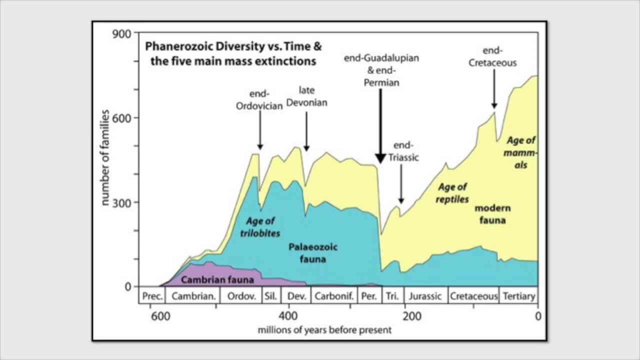 So occasionally we have some good news to spread, But species are dying out at an incredibly fast rate, so fast, in fact, that it's basically matching some of the major extinction events in the history of the Earth, And there's been five of those. 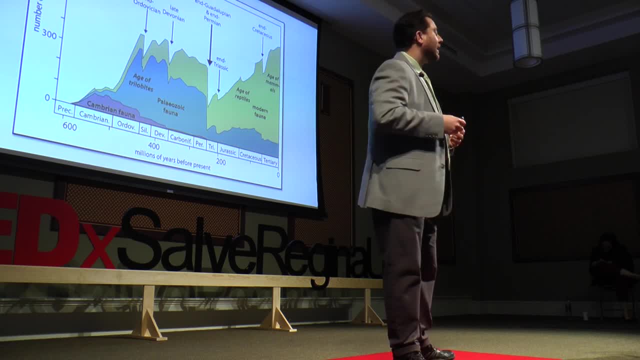 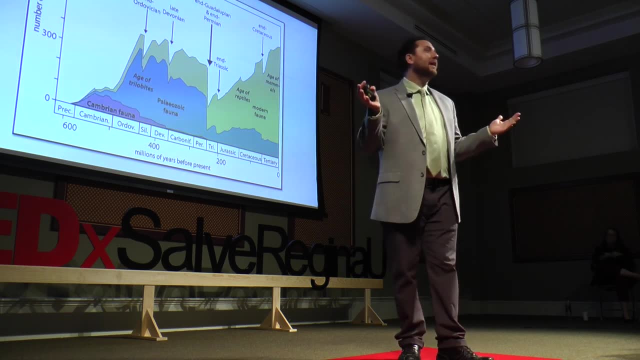 The most famous of those events was the last one. that happened at the end of the Cretaceous period. This is when this giant asteroid hit in the Yucatan Peninsula and basically ended the age of the dinosaurs, So this is the one that we're most familiar with. 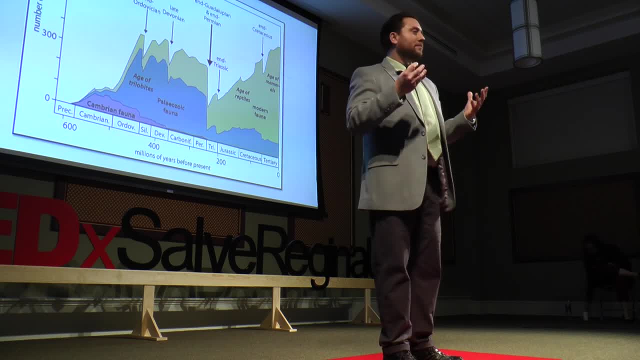 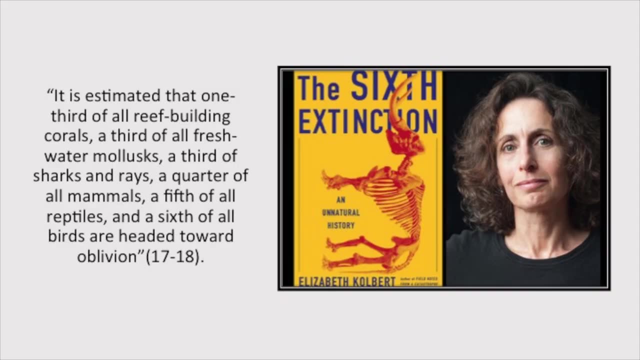 That was the fifth mass extinction. It's pretty clear now to most scientists that we are right now in the midst of the sixth mass extinction In 2014,. Elizabeth Colbert from The New Yorker wrote a book called The Sixth Extinction. It's an incredible book. 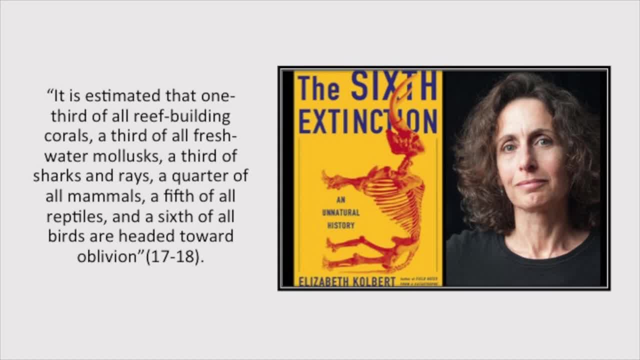 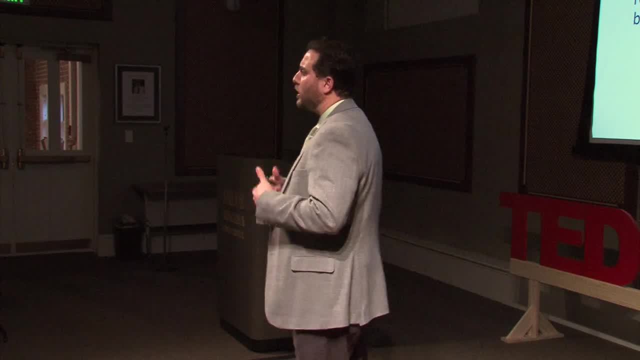 Again, not exactly a cheery one, but an incredible book, in the sense that each chapter is devoted to a particular species that either gone extinct or is on the verge of extinction, and drawing upon the scientists who are really close to the ground with these various species. 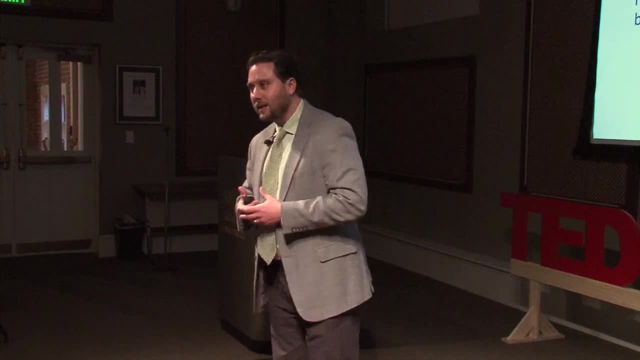 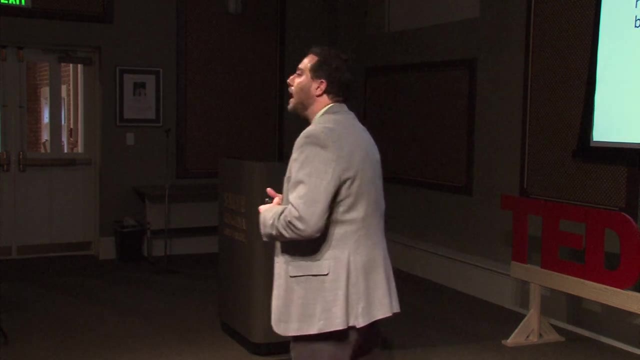 And basically the consensus is that species have always gone extinct throughout the Earth's history. But if you compare the background extinction rate to the rate of extinction today, it's almost undeniable that we're in the midst of the sixth mass extinction. Why is that? 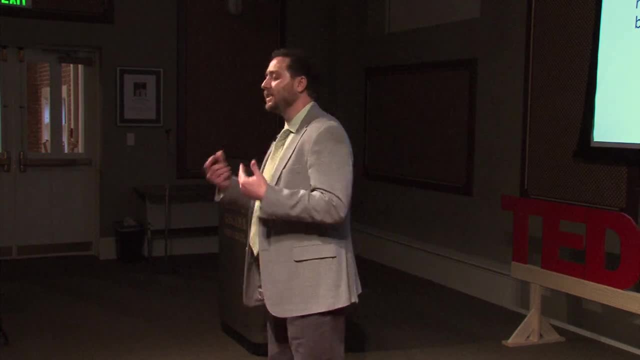 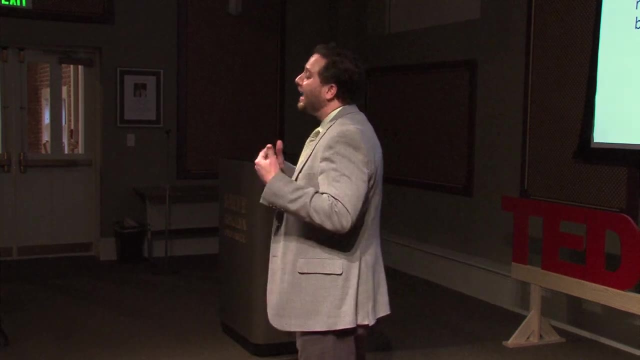 Well, it's a combination of factors: It's global warming, it's the acidification of oceans, it's deforestation, it's invasive species, it's overhunting, it's poaching, it's a lot of things. But all of those things, by the way, come back to us. 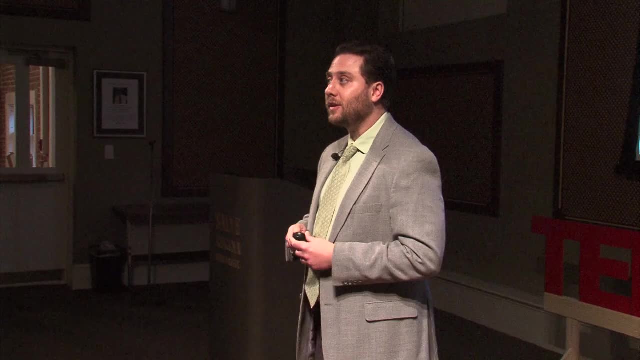 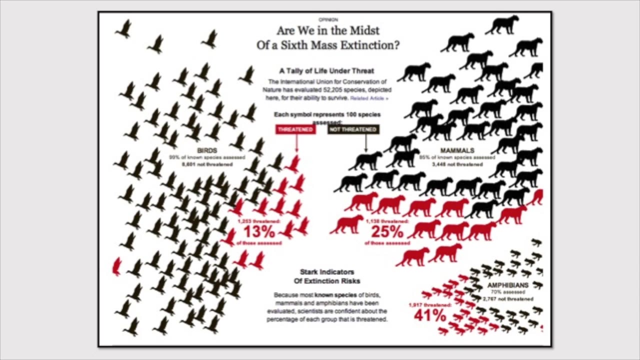 We are causing the sixth mass extinction in the Earth's history. Again, not exactly great news If we look at where things are going, moving forward. this is an image from The New York Times from a couple of years ago. Roughly a quarter of all mammals are endangered. 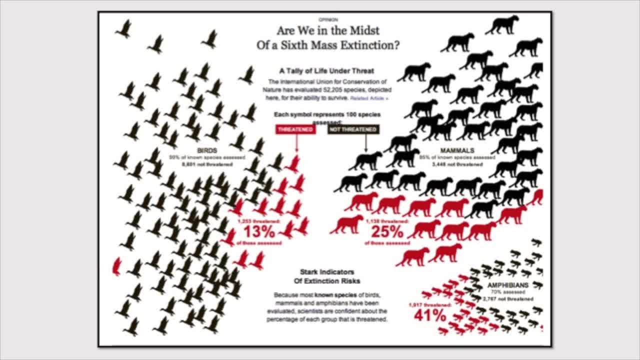 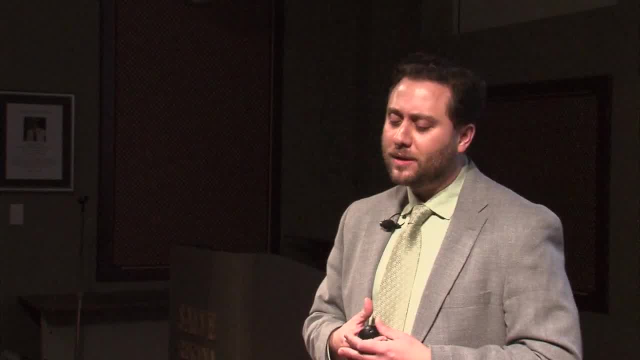 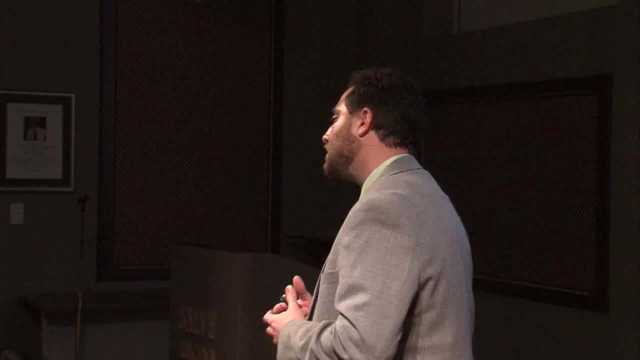 At this point. you see, amphibians are actually doing much worse. 41% of amphibians are thought to be endangered at this point. One of the chapters in Colbert's book is devoted to amphibians in the Amazon rainforest, which are dying off in huge numbers because of a fungicide that's actually killing them off. 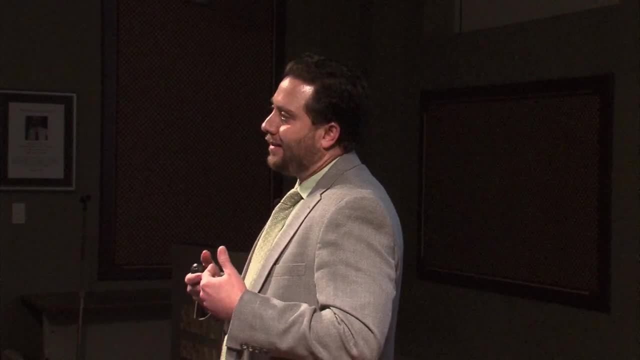 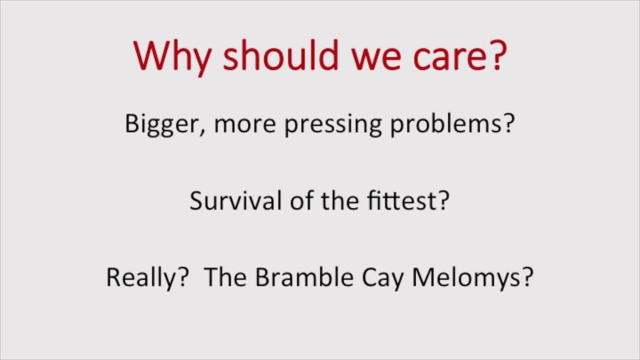 at a quite rapid rate. So what do we do with this? The big question that I want to talk about today is: well, why should we kill them? Well, why should we care? I'm not going to address all of these questions today, but one of the things that a lot of 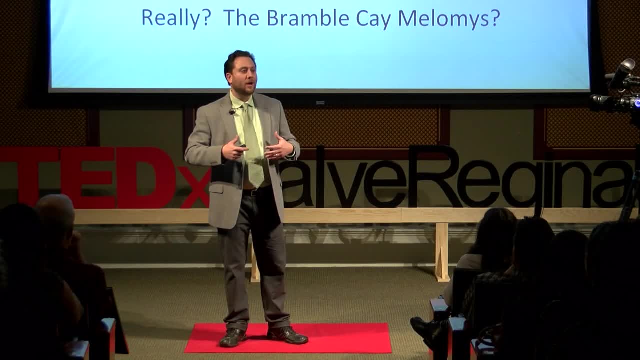 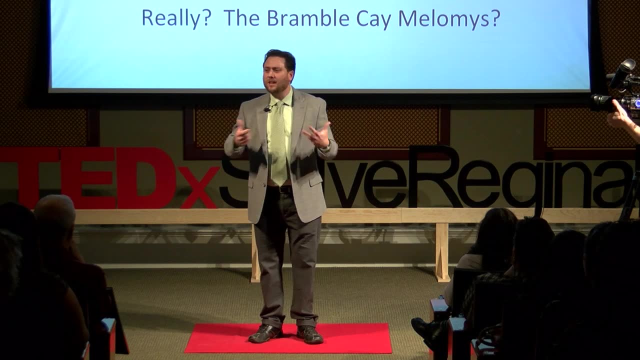 people say in the face of species extinction is: well, aren't there bigger problems? Aren't there more pressing problems? What about human beings who are suffering? How do we basically align, or how do we make sense of where our priorities lie? 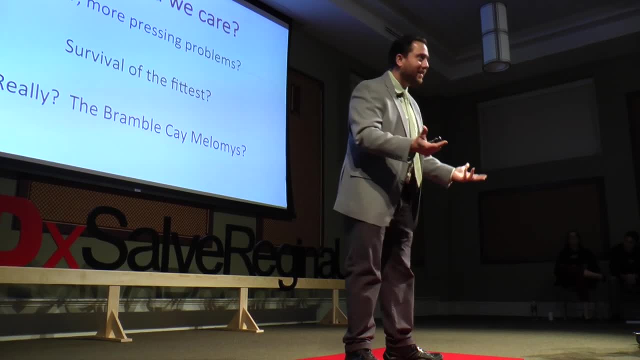 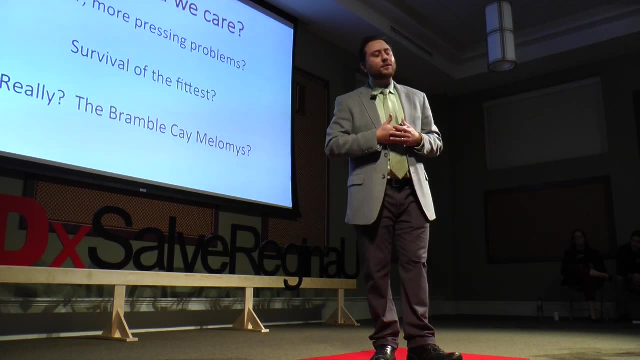 Others might say, hey, survival of the fittest, We're the fittest, We won. So if other species are dying off, they just weren't strong enough. Can we spin it that way And maybe we don't feel quite as badly about ourselves? 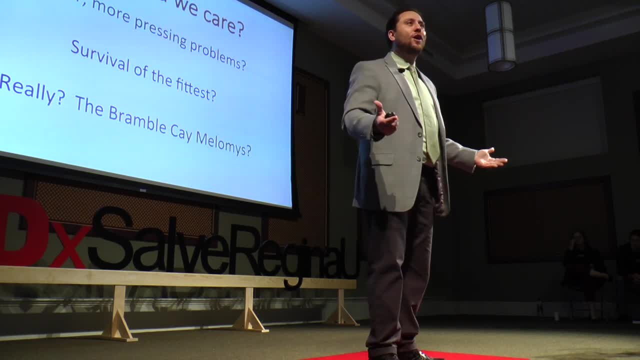 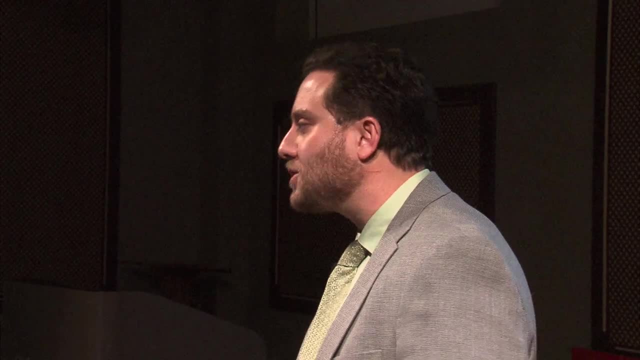 And really the Bramble Cay Melamese. nobody heard of this five minutes ago, so you're asking me to care about something that I never heard of before. Why should I care? I think the easiest argument to make is to say: this comes back to bite us in the end. 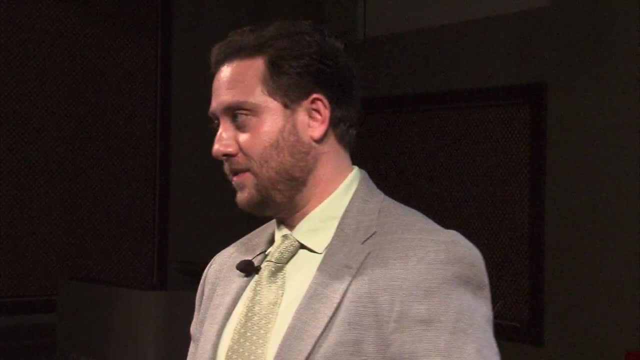 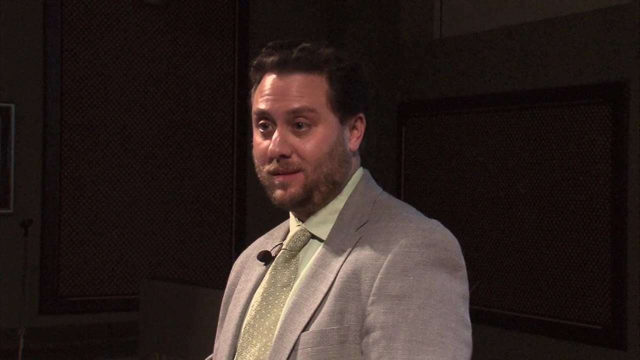 and it's already doing so, Whether we're talking about interruptions to the food chain, ecotourism, how ecosystems are being thrown off by removing one species, And maybe we're going to get rid of one species, And maybe we're going to get rid of another species. 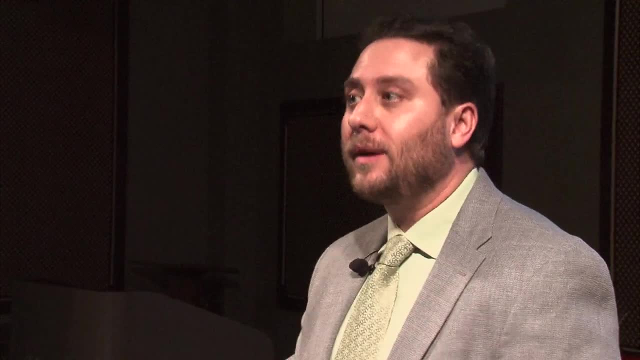 And the basis for this argument is the timelines. The Chinese have often introduced a foreign, invasive one, And human beings are suffering directly because of this, And I think that's the easier argument to make. Philosophers refer to this as the anthropocentric argument. 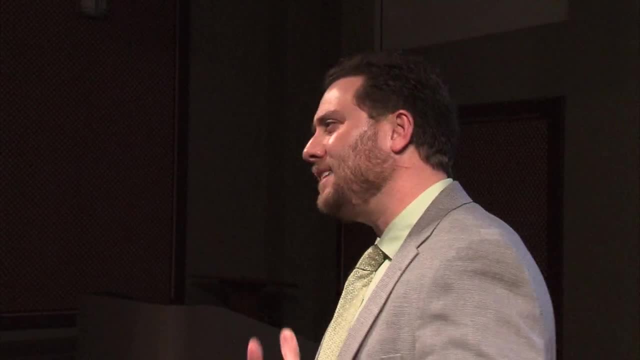 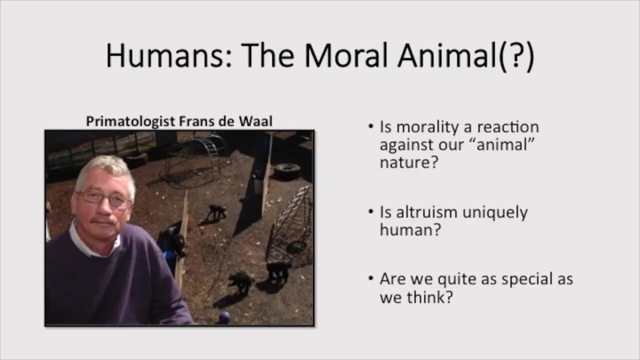 But I think there's a higher level argument that we can make here that appeals to something that's unique about us as human beings: Franz De Walle. he's a primatologist, works out of Emory University, and he spent most of his life studying other primates- chimpanzees, bonobos. 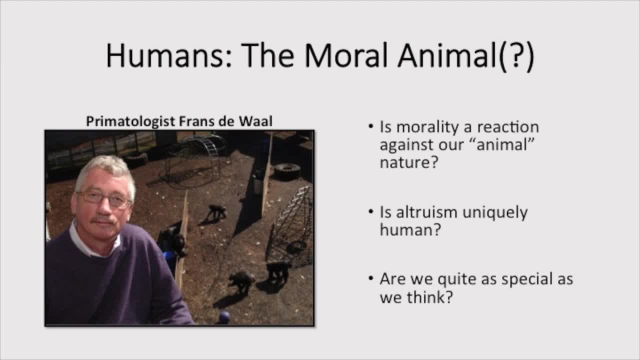 And the last 20 years or so, he's been making the argument for a long period of time, about making the argument that our closest genetic relatives are much more social, dare we say even moral, than we've traditionally given them credit for Philosophers throughout history. 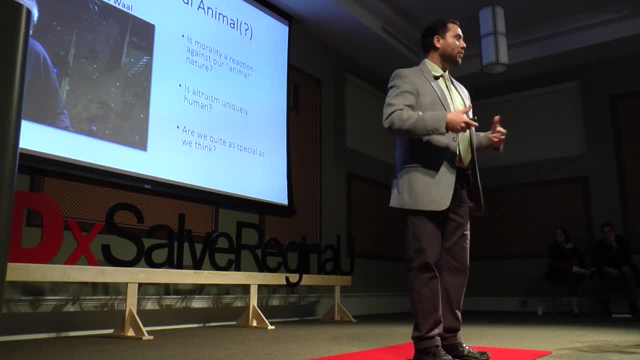 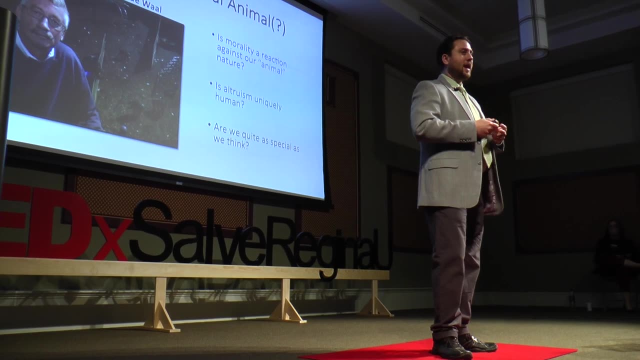 at least in the Western tradition, have spoken of ethics as overcoming our animal nature, and De Waal thinks that that's completely unfair, because animals, especially those closely related to us, are quite social and they oftentimes exhibit behaviors that are pretty identifiable to us. 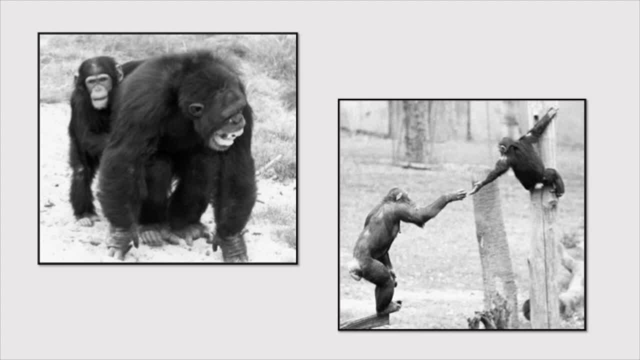 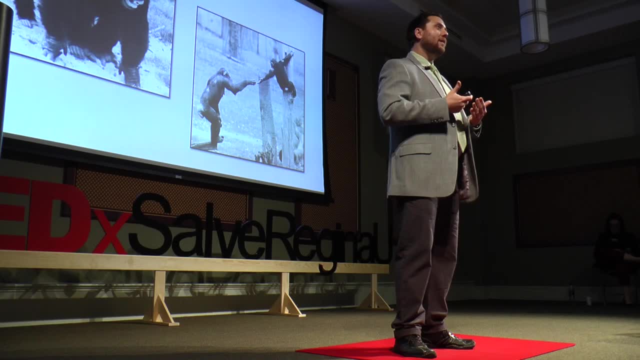 consolation behaviors, altruism, even sometimes a sense of justice, And what he wants to say is that there's a moral continuity here and that we shouldn't be surprised by that, because we're 98% similar. So to think that all of a sudden human beings showed up. 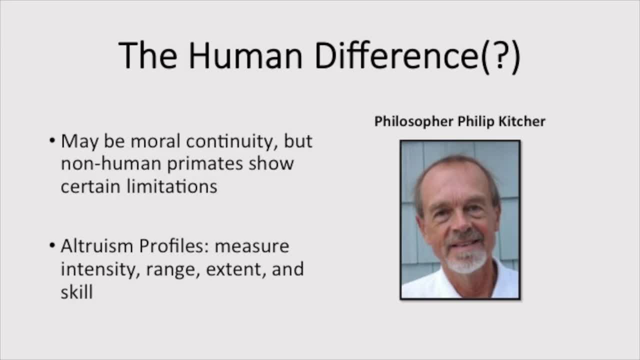 and were uniquely moral. he thinks that gets it wrong. Now, even if we acknowledge that moral continuity, Philip Kitcher, a philosopher at Columbia University, says there must be something that's different about humans. There must be something different about human beings. 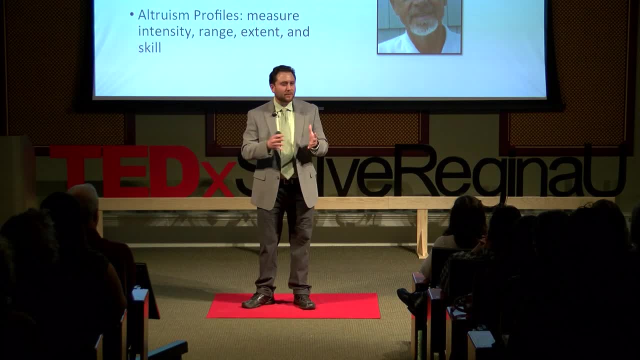 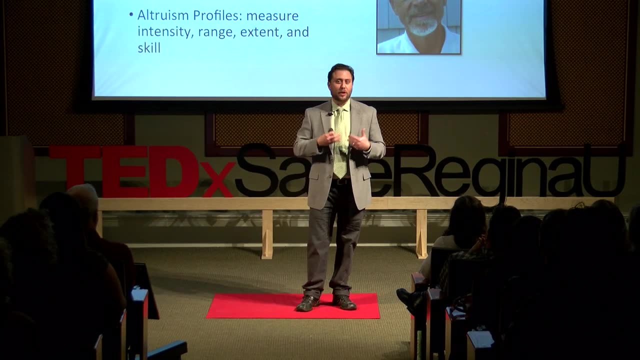 right that we could acknowledge this continuity, but there seems to be some kind of break, some kind of difference, And what he suggests is drawing what he calls altruism profiles, which basically say: well, how far are we willing to go to help out people who are unlike us, who are strangers? 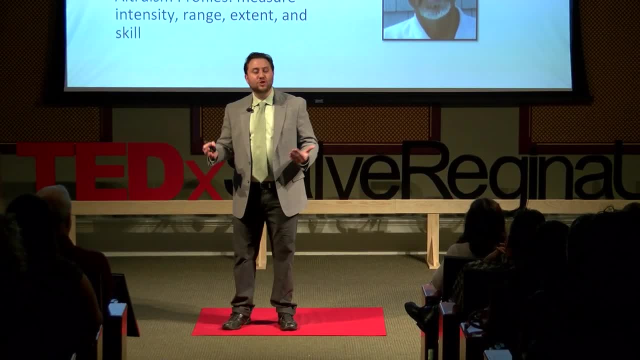 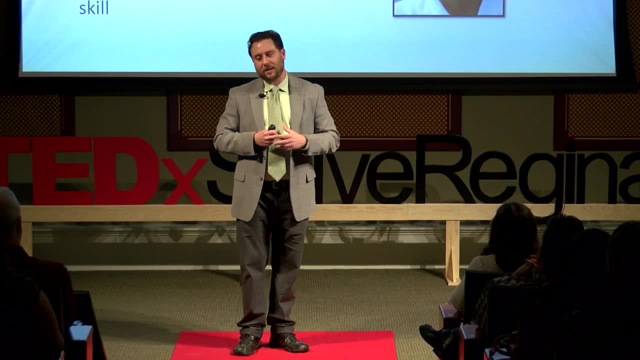 right, who we have no immediate sort of relationship with, at least familiarly right, And he suspects that well, we might see these sort of proto-moral behaviors in other primates. but it seems like human beings are capable, and have oftentimes gone further, in helping. 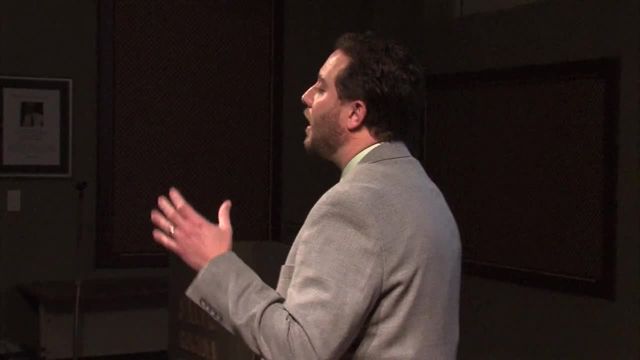 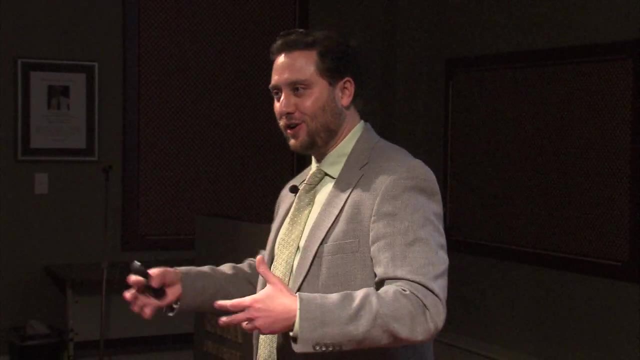 out those who are quite unlike themselves. okay, I think Kitcher's probably right about this. You know, if you've ever watched your nature specials on, you know your planet Earth or your NOVA specials, you know chimpanzees can be terrifying. 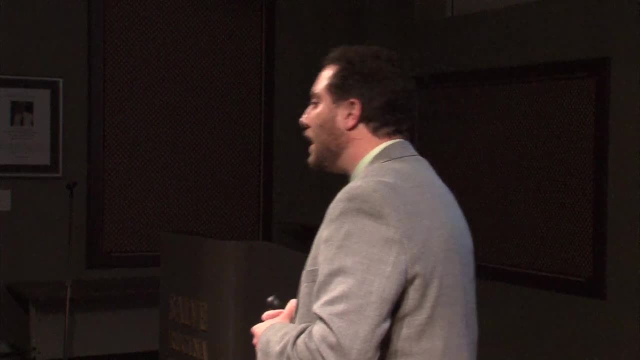 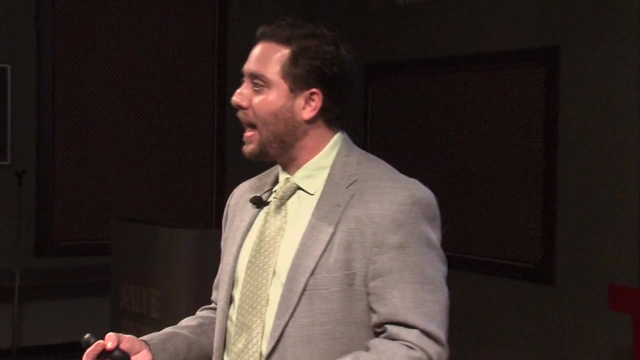 especially to members outside of their group, And human beings, at least when we're at our best, seem to be capable of doing much more than that, But of course we also know that at our worst we're just as bad right. 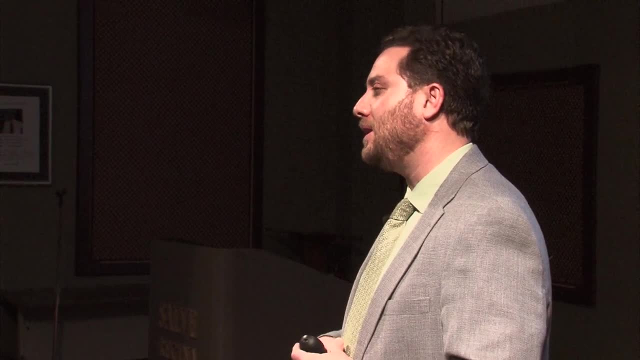 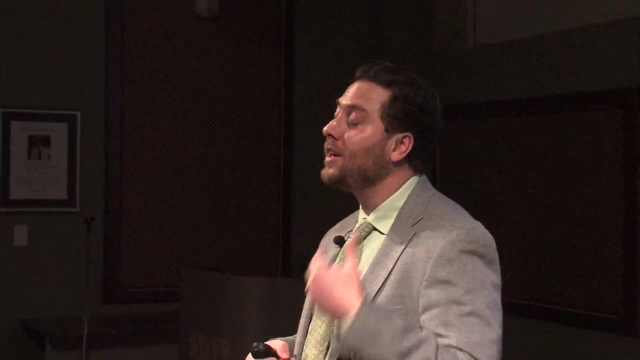 So if we really want to say, why should we care about the distinction of these species? perhaps we need to call upon sort of a higher moral capacity that human beings may in fact be uniquely capable of, even if we don't quite exercise as much as we should. 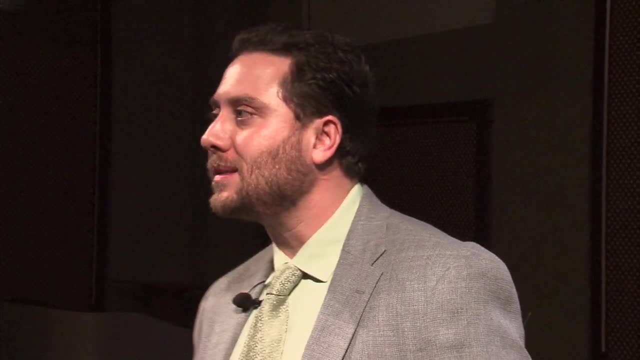 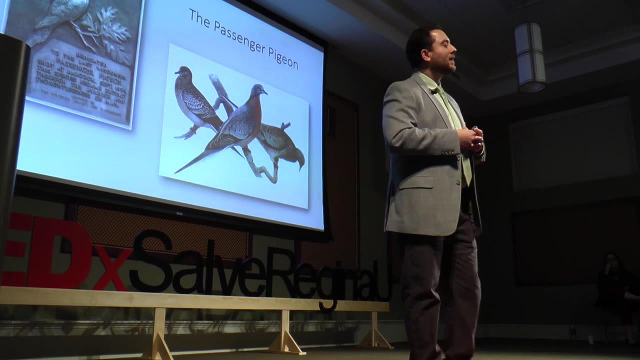 This brings me back to my initial point about the Bramble Cay Melanies. Aldo Leopold, some of you may be familiar with, is usually thought of as being the father of American conservation, His Sand County Almanac published way back in 1940,. 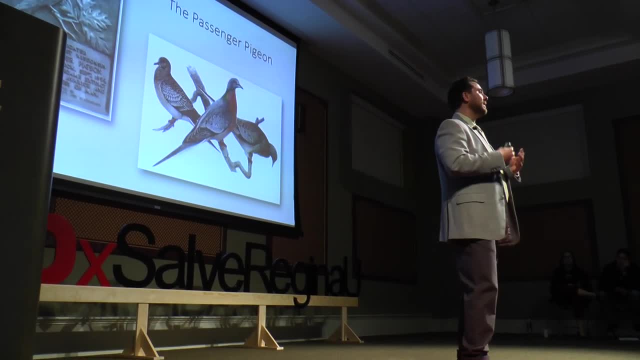 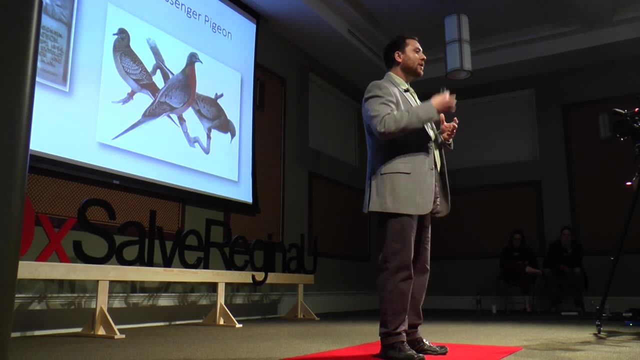 1949, is still widely read and used by conservationists, by philosophers, by people who just love nature and the environment. And he spends a long section of this book talking about the passenger pigeon. And the passenger pigeon is a species that more or less 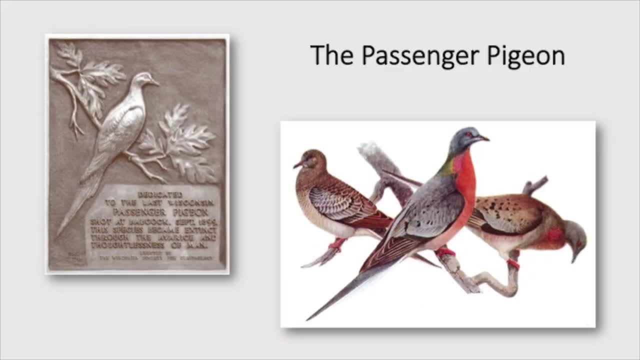 we hunted to extinction. And he reflects on this monument that's erected to the passenger pigeon in great sadness at the loss of this species. And what always kind of strikes me when I read this to my students is they, you know, they never really heard. 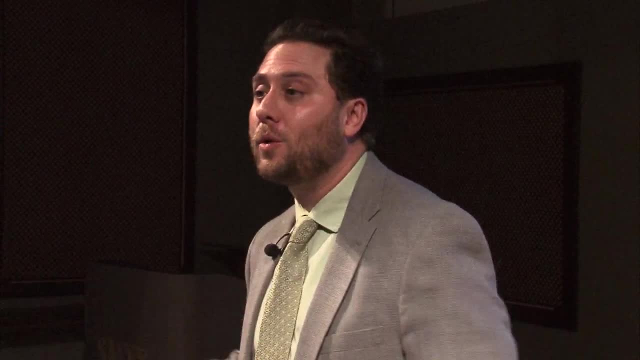 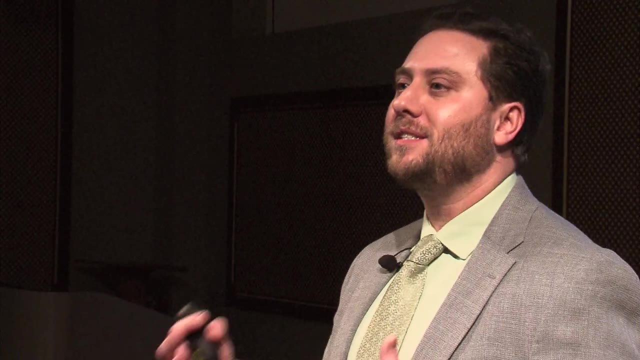 or maybe they'd heard of the passenger pigeon but they didn't know it had gone extinct and they certainly didn't know what it looked like. And this is kind of news to them, even though it's from 100 years ago. And this is where I see the similarity with the Bramble Cay Melanies. 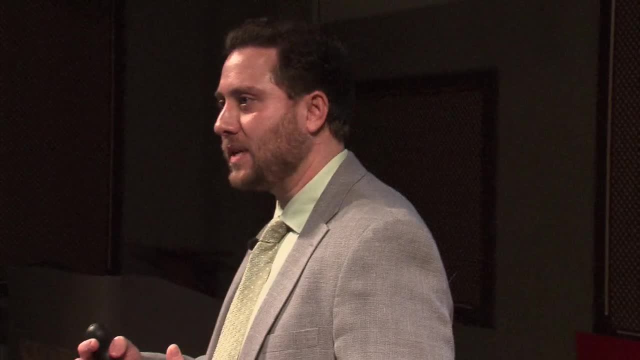 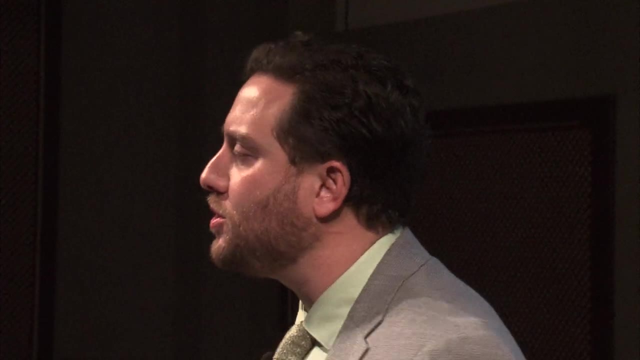 is that maybe the first point is just to kind of notice what's happening and to realize that something's being lost here. that again, if we're true to who we are as human beings, maybe it should bother us, Maybe it should impact us. 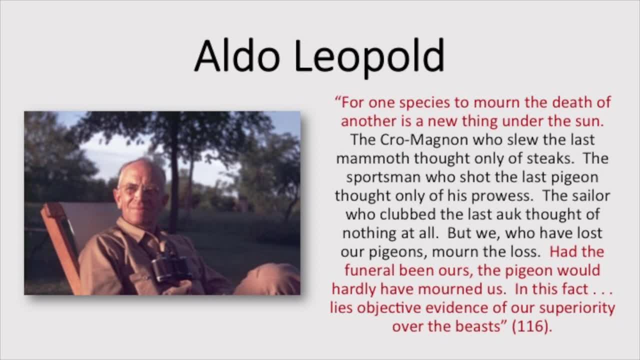 And I want to include this really powerful passage from Leopold right That, in reflecting on the loss of the passenger pigeon again, which a lot of my students had never heard of before they started reading about this, He says that for one species to mourn the death,